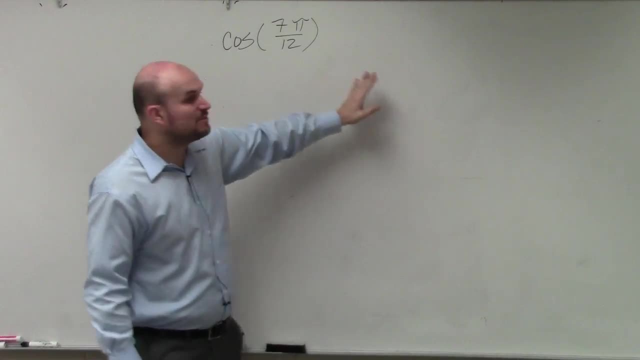 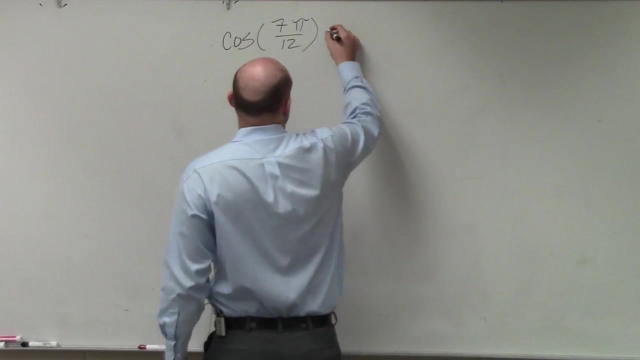 Or at least 7 pi over 12.. So what we can do is we want to say: can we break this up into the sum or difference of two angles? And what I did was I was trying to help you guys out and I said: guess what guys? 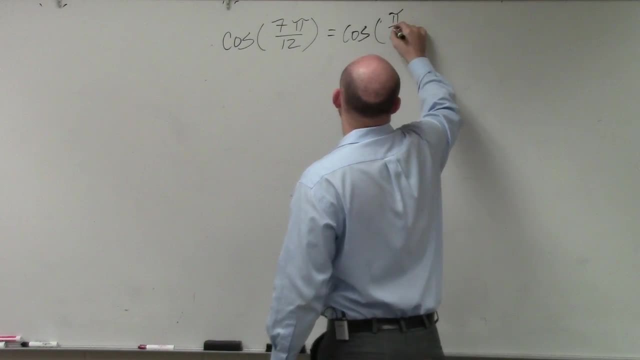 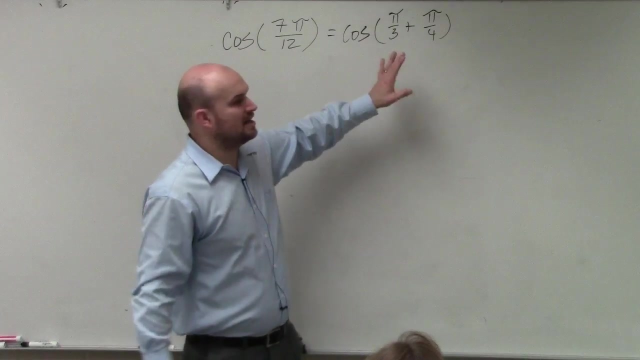 We can. We can break this up into the cosine of pi over 3 plus pi over 4.. Right, This is what I told you guys to say. Hey, I'm going to help you guys out. I'll break these up for you guys. 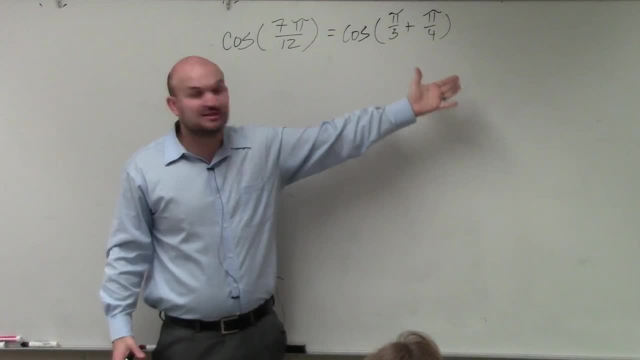 So the pi over 3 plus pi over 4, if you get common denominators- ends up being 7 pi over 12.. And you can do your math on the side if you'd like to, But that's the angle broken up. 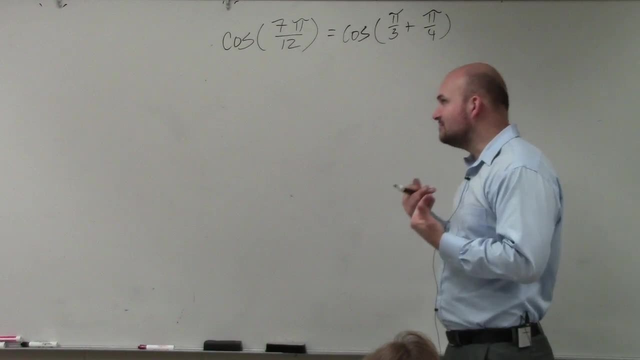 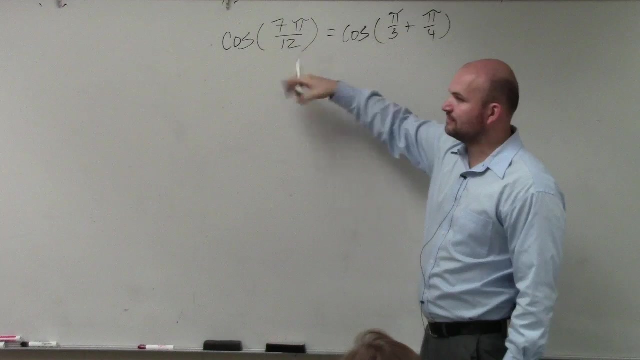 Huh. How did you come up with that? Who's knew it? I told you you don't need to worry about doing this. That's why I gave you this answer at the end of class. I don't really need you to think through this. 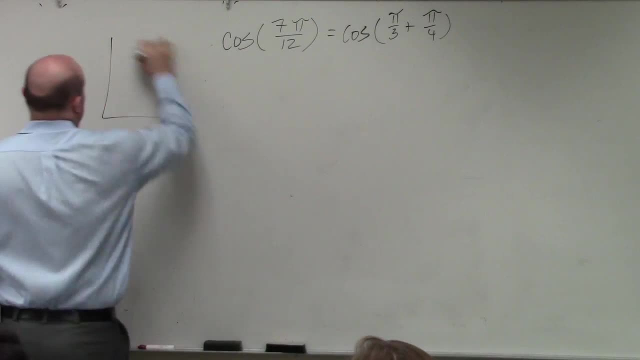 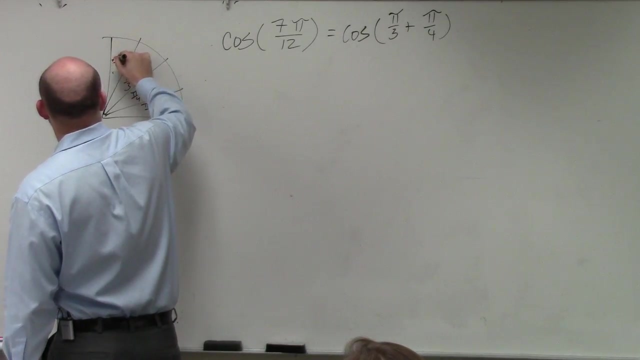 But I mean, there's only so many angles that we've talked about. So you have pi over 6,, pi over 4,, pi over 3, and basically pi halves. You're not even going to use pi halves, but we could say it. 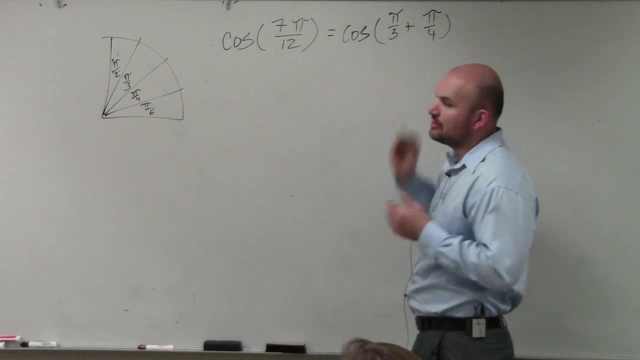 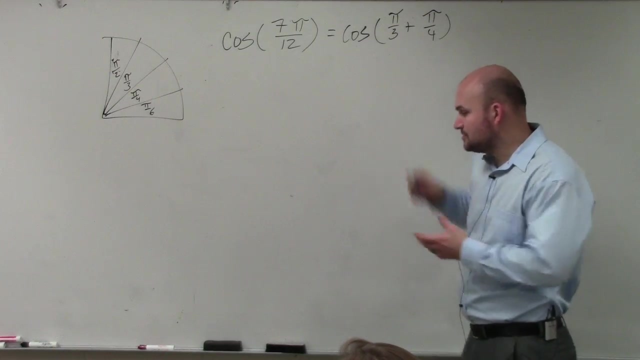 Well, basically adding those four, Or adding or subtracting, how can you get to 7, pi over 12?? Well, remember, to combine them, you have to have common denominators, right? So it's just my intuition knowing: hey, to get common denominators, I need to multiply by 4 over 4 and 3 over 3.. 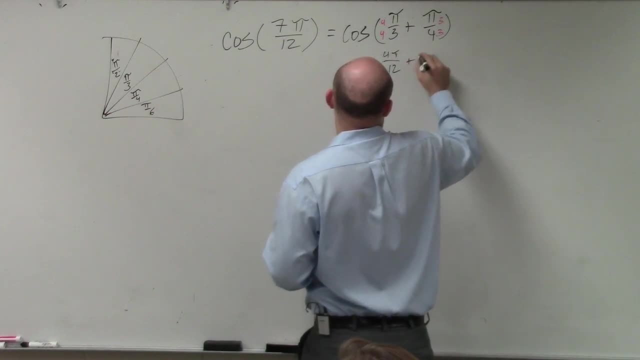 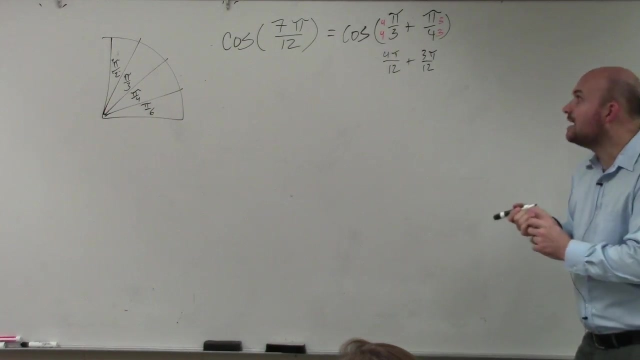 Correct, So this would be 4 pi over 12 plus 3 pi over 12.. Do you now see how those add to give you 7 pi over 12? Right, I mean, there's only so many options you can break this apart into. 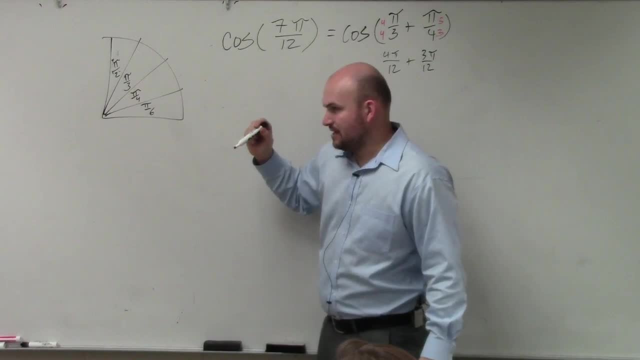 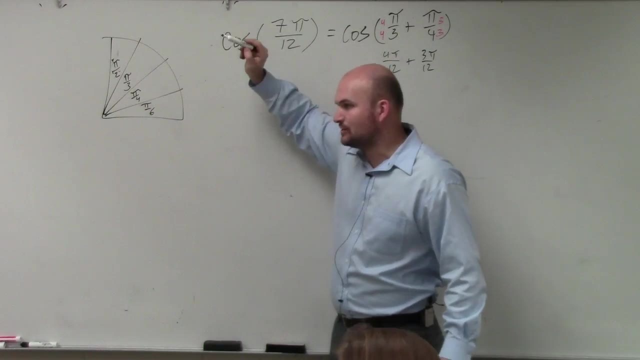 You have to break it up into one of these angles, right? You don't want to break it up into 10 pi over 12 and 1 pi over 12, because those are not angles that have coordinate points on the unit of circle. 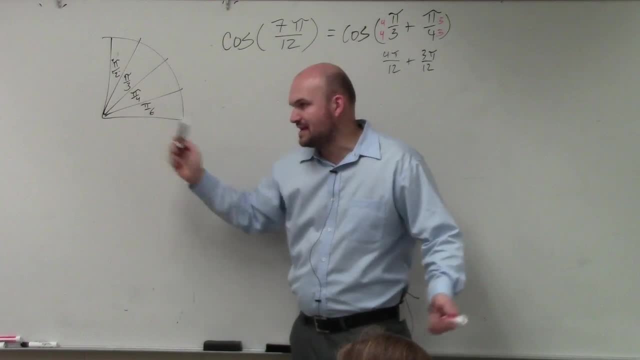 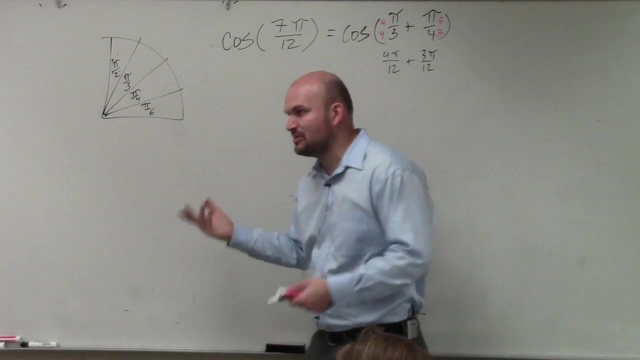 So you can only work with these angles, You can only add and subtract those angles, So you can guess and check, or once you start getting some practice it'll start coming a lot easier. I know degrees is much easier, right Like you have 15 degrees. 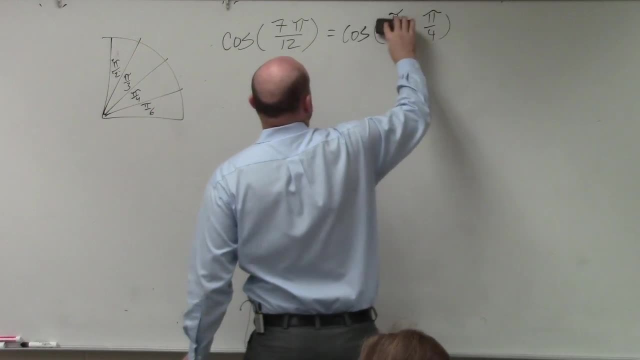 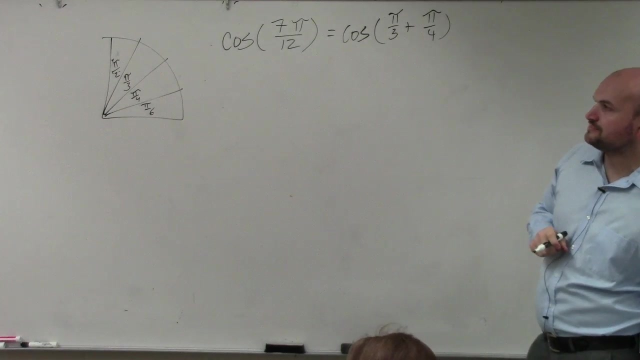 Oh, that's 45 minus 30. But I didn't want you to be, I didn't want you to get stuck on this. that's why I gave you the solution, Or at least the angle broken up. Can't we just change it to degrees? 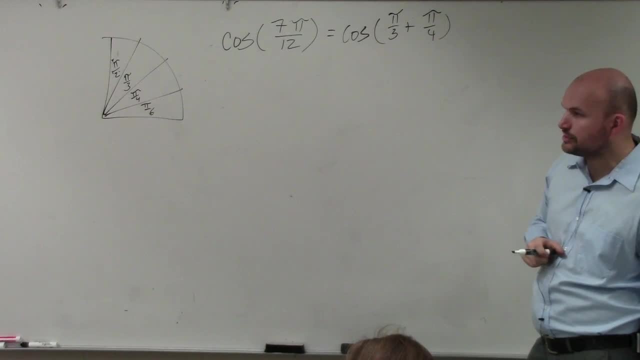 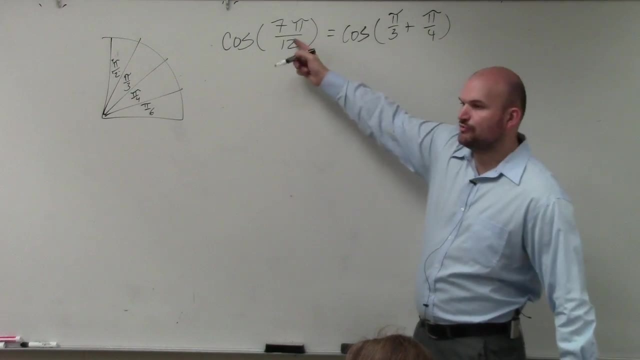 You could. you could also do that. If you're really having trouble, you can just break it into degrees and then figure it out Absolutely. So, this would be 60 degrees plus 40 degrees, right? Or break this up, convert that to degrees and say: you know what would that be? 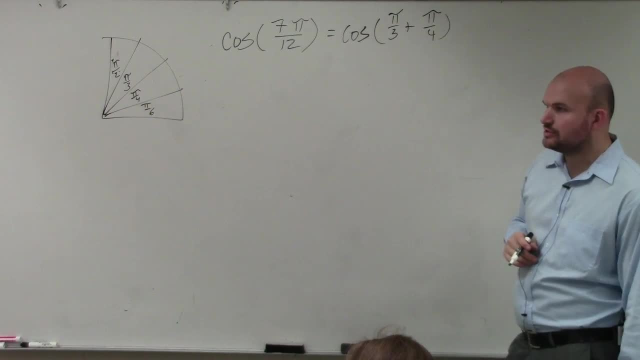 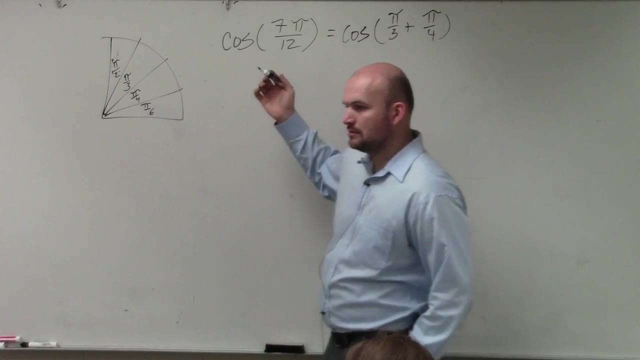 Right. So 60 plus 40 would be 95 degrees, Right. So, yeah, you can do that as well. It's another option. Yes, You understand that. Breaking degrees. Okay, Wouldn't that be like 105?? Yes, 105.. 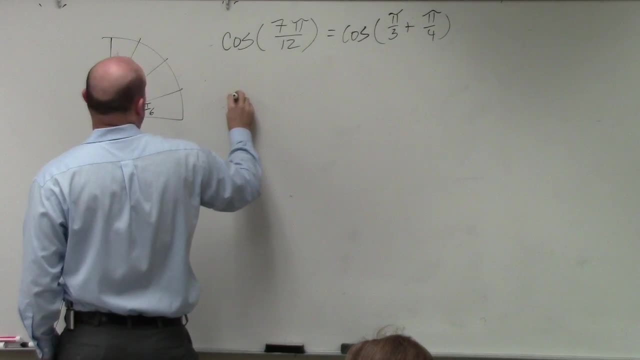 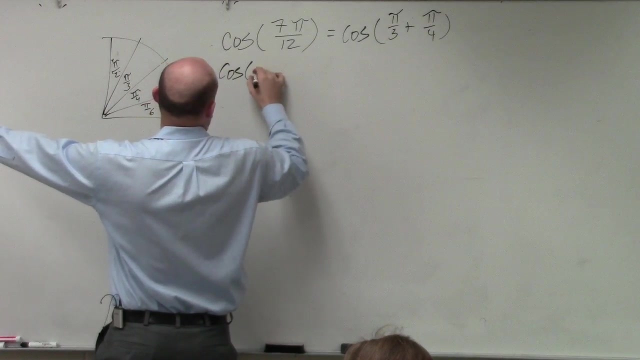 Yeah, 65.. Yeah, thank you. So now we're going to do cosine. So you can see, this is the addition. So I'm going to use the cosine formula for addition. So by following the cosine of u plus v, if you guys look at my formula. 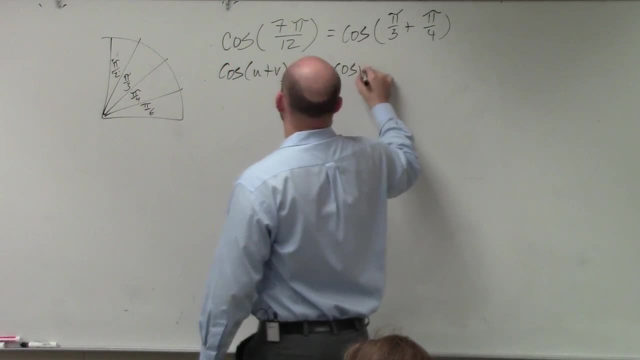 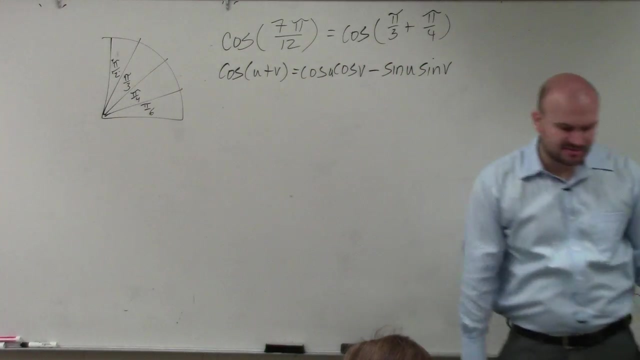 which you will be provided, is cosine of u times cosine of v. Notice how the sine switches, Then goes to sine of u times sine of v. Whenever I'm doing these problems, the best thing I like to do for these guys is I like to identify. 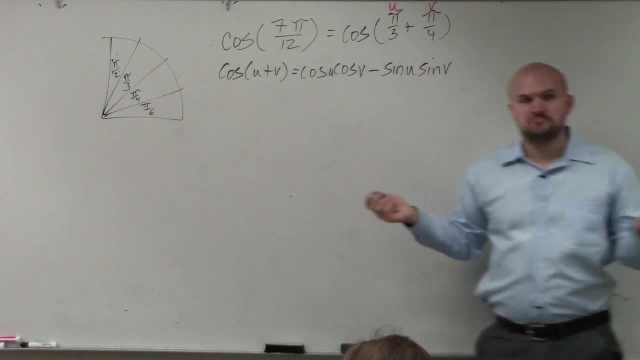 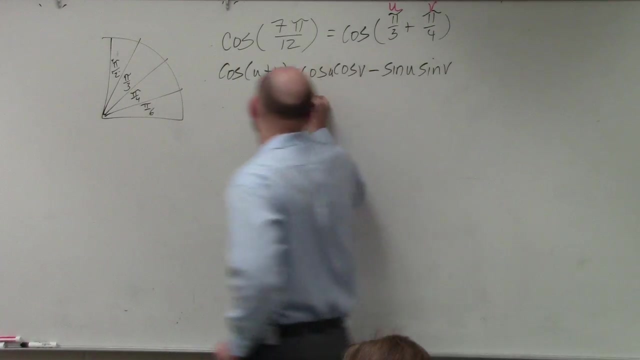 I like to identify my u and I like to identify my v. Okay, Doesn't really matter, Justin, You just want to make sure you identify your u and your v, And then you basically plug them in. So I have the cosine of pi over 3 times the cosine of pi over 4. 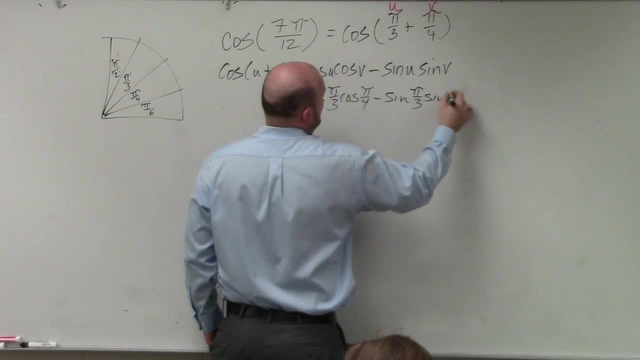 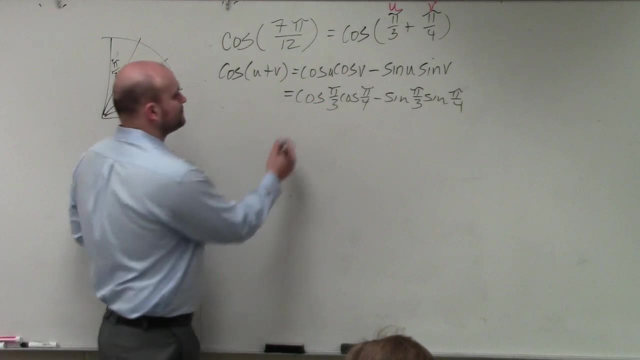 minus the sine of pi over 3 times the sine of pi over 4.. All right, Now we just go ahead and evaluate using our unit circle. I'm going to do this rather quickly because I'm assuming you guys can find it All right. 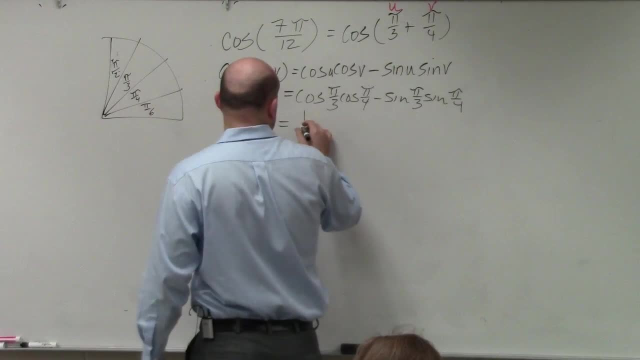 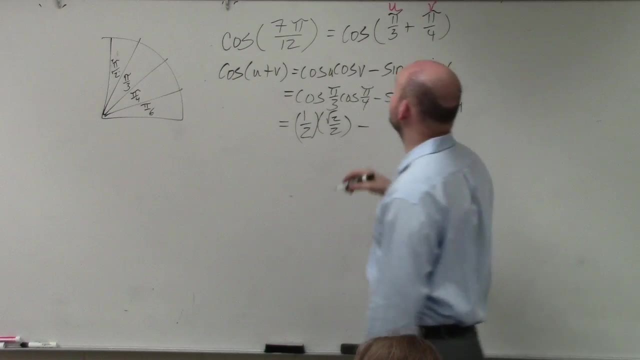 You can follow along like that with me. The cosine of pi over 3 is going to be 1 half times square root of 2 over 2, minus the sine of pi over 3, which is going to be square root of 3 over 2,. 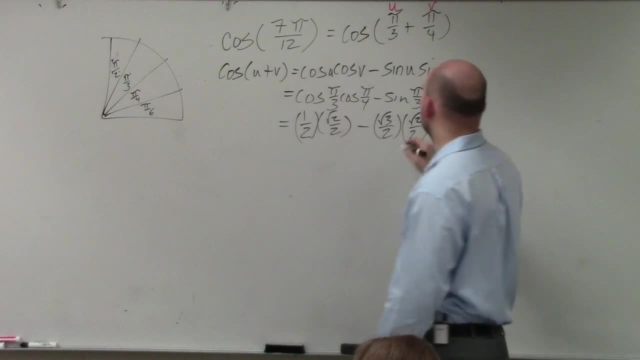 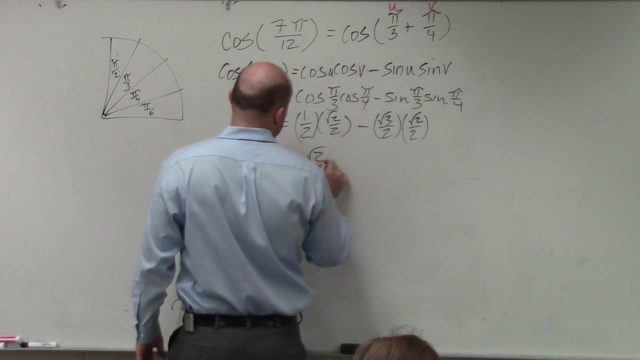 and the sine of pi over 4, which is square root of 2 over 2.. Does everybody follow Points? And then we just multiply and simplify. So I have square root of 2 over 4, minus the square root of 6 over 4.. 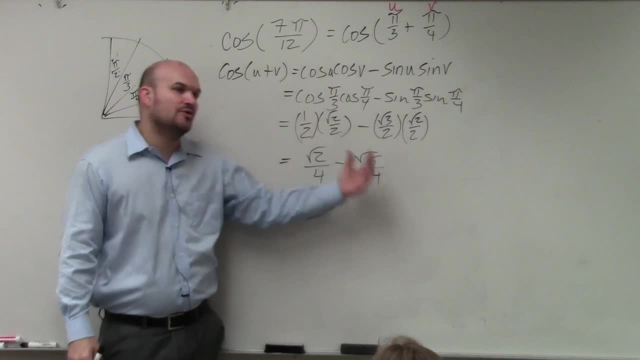 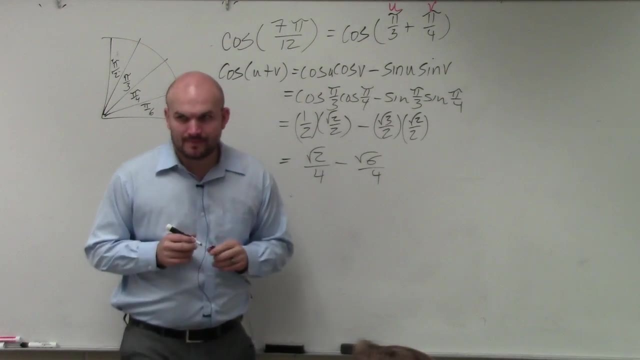 Again, you can leave your answer like that. You can combine them with the same denominator, or you could factor out a term. I'll just leave it like that to keep the answer simple. We're going to do a tangent today in class, anyways. because I know you guys need more help with that.